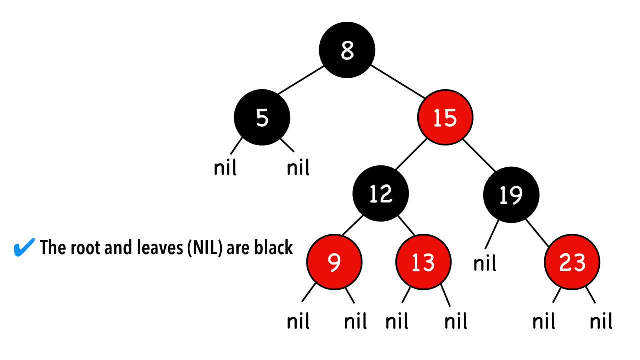 The root, node 8, and all nil nodes are black. All red nodes have black children. Lastly, all paths from a given node to its nil descendants contain the same number of black nodes. Let's use the root as our given node. 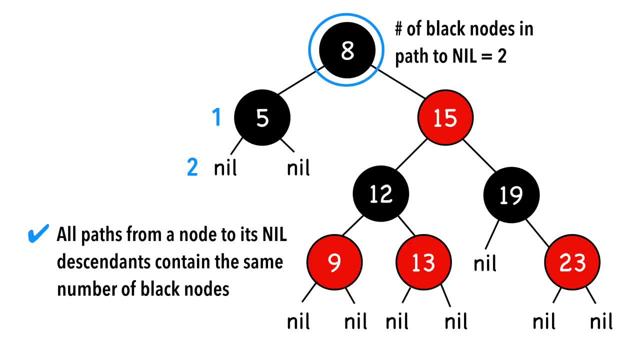 node. We see that all simple paths to nil nodes contain two black nodes. One note here: when counting the black nodes in our path we don't count the starting node. We call this number 2, the black height of the red black tree. That is the number of black nodes from the root to the 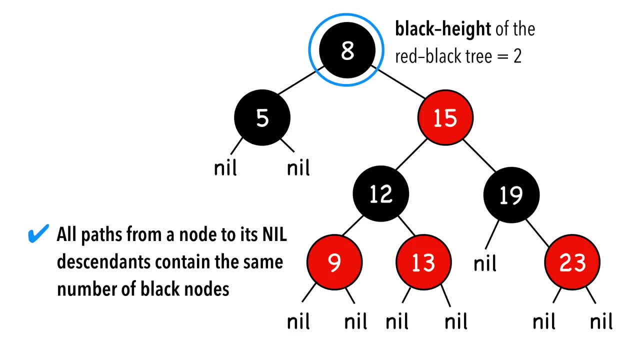 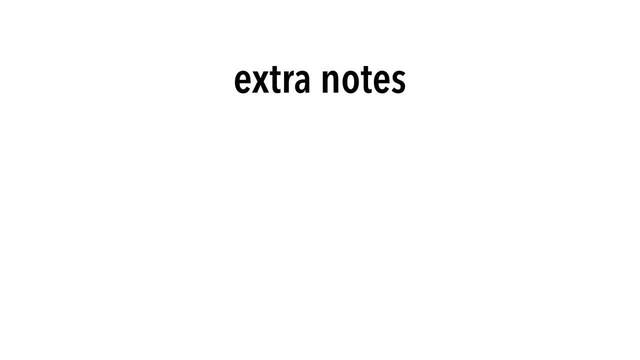 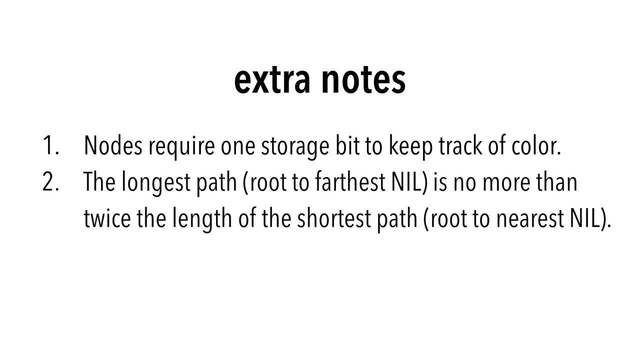 nil nodes, not counting the root itself. In fact, each node has its own black height. A few notes before we finish. Nodes require one storage bit to keep track of color. Second, the longest path, that is the path from the root to the farthest nil. 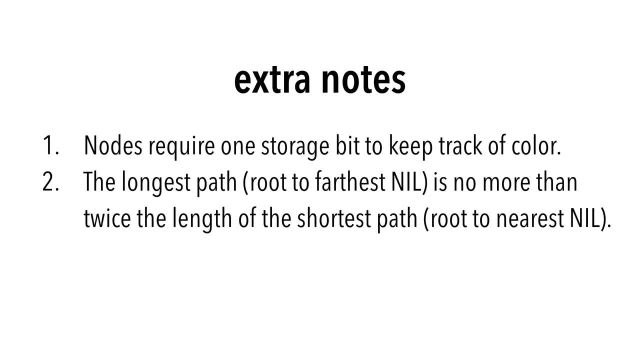 is no more than twice as long as the shortest path, which is the path from root to the nearest nil. In other words, the shortest path has all black nodes and the longest path alternates between red and black. This is because of the constraints we defined earlier. 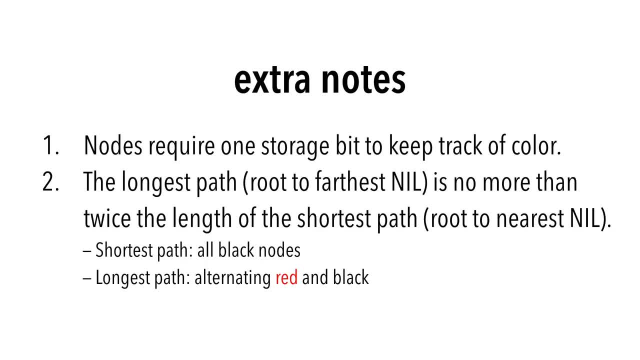 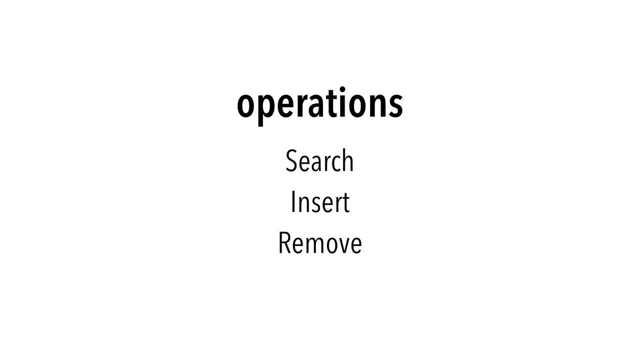 take a look back at our example and you'll see. So how do we use red black trees Just like any other binary search tree. there are three main operations: Search, insert and remove. Searching is no different, but inserting and removing nodes require rotation because we must maintain the properties of red. 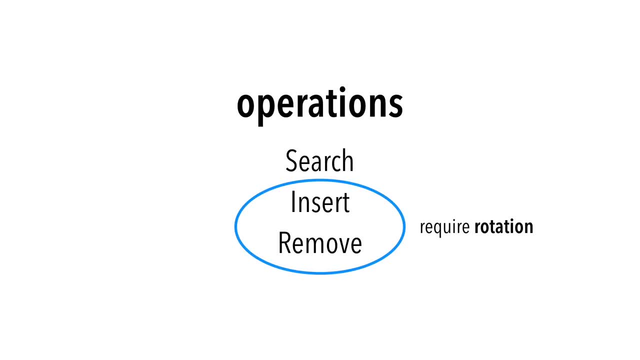 black trees. We'll cover these two operations, as well as rotations, in future videos. These operations have a time complexity of big O of log n. As we said, the maximum height of the tree is on the order of log n. Finally, because we only require one extra storage. 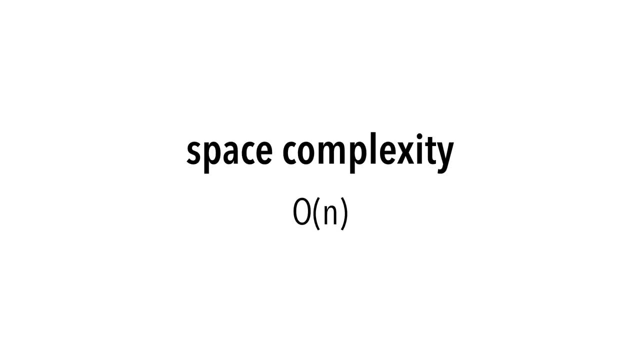 bit. the space complexity is big O of n. Thank you for watching. Stay tuned for more videos covering red black trees. Please like and subscribe if you enjoyed the video.